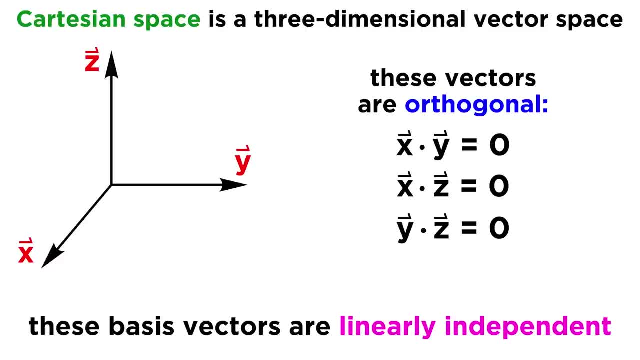 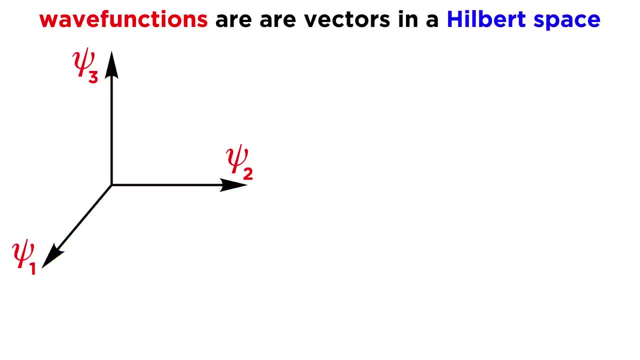 These basis vectors are linearly independent, so we can't write any of them in terms of the others, since no combination of x and y can give us the z vector and so forth. Now back to wavefunctions. Each wavefunction is a vector in a Hilbert space, just like. 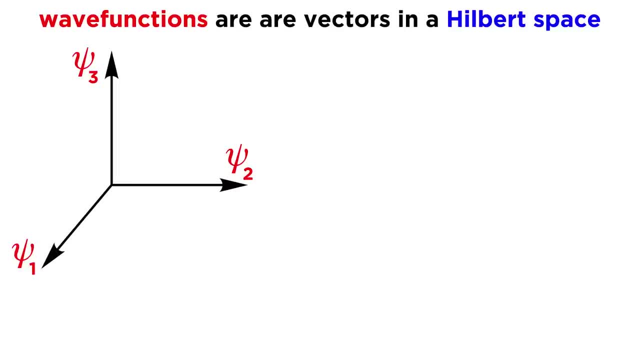 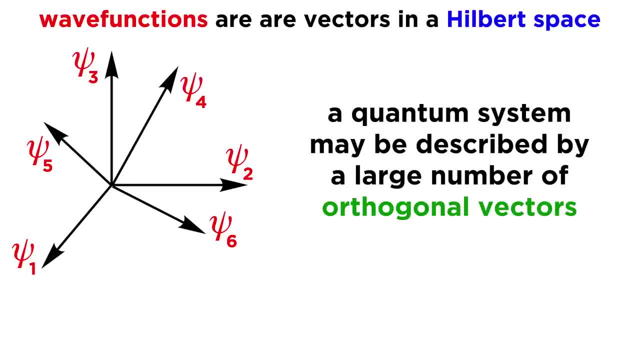 space. x, y and z are vectors of the same vector, space. The difference is that a quantum system may be described by a large number of wavefunctions, much more than three, all of which are orthogonal with each other, and they are also linearly independent meaning. 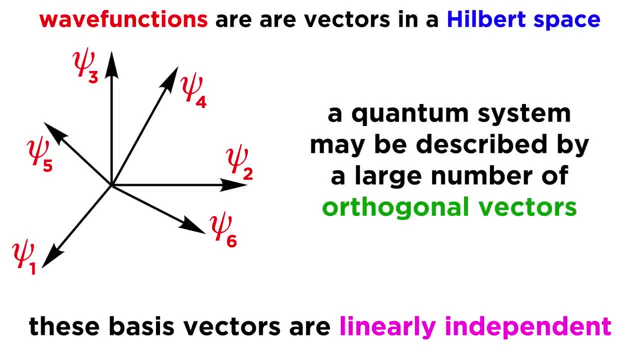 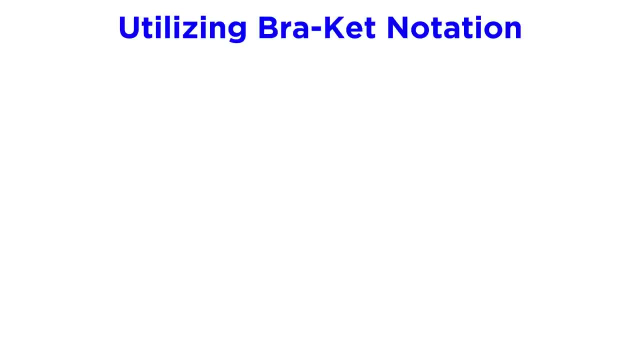 that none of them can be written in terms of the others, just like in the three-dimensional case. Now that we are conceiving of wavefunctions as vectors, it's time to introduce some some new notation: braket notation. This notation utilizes two constructs: bras and kets. These 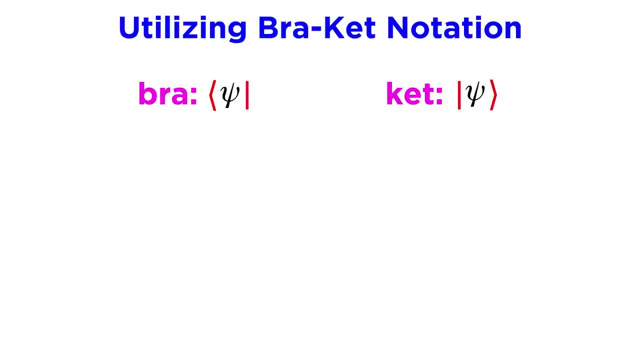 use angle brackets and vertical lines to represent certain vectors, and we will use this notation with the wavefunction When we use a ket. this way, we are referring to the wavefunction in vector form, where a, b and c can be considered coefficients that accompany each component. 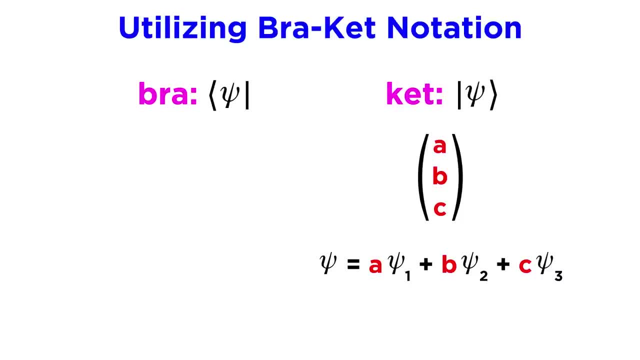 of that wavefunction no different from how we've used vectors to represent functions in linear algebra. So psi equals a, psi one plus b, psi two plus c, psi three, with each of these representing basis vectors. This represents the sets of linearly independent. 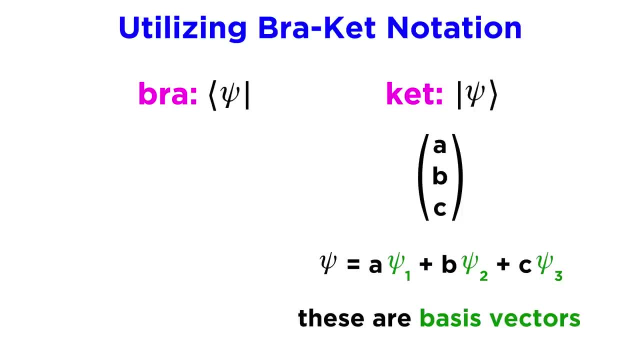 wavefunctions that are solutions of the system. So, once again, considering the ket to be a shorthand for the vector representation of this wavefunction, we're going to have to use a new notation: the bra can be considered the complex conjugate of the ket or psi star. 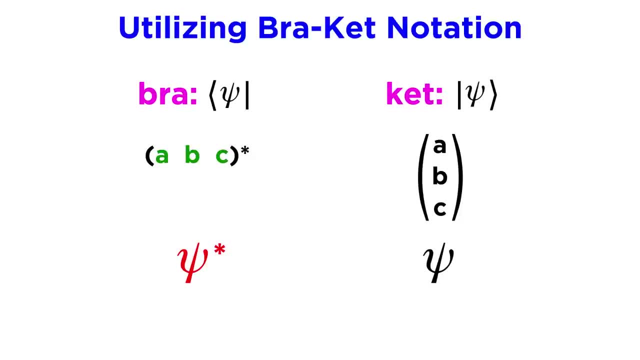 which is the transposed conjugate of this vector, therefore involving a, b and c, arranged in a row instead of a column, and with a star indicating that each term is the complex conjugate of its corresponding term in the ket, or a star, b star, c star. Now we are ready to. 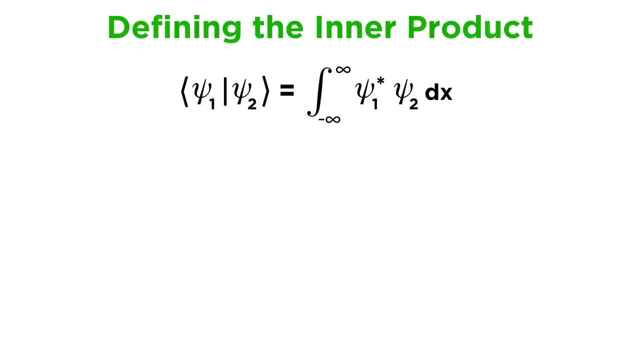 define a new operation. We're going to use a new operation called the inner product. in a Hilbert space which uses the bra-ket notation we just learned, The inner product of psi one and psi two is equal to the integral over all space of psi one star times psi two with respect to x. 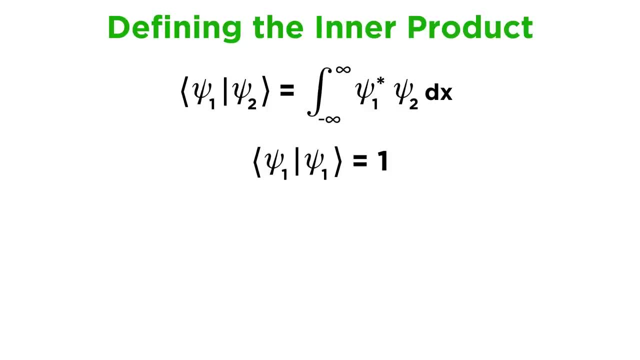 A few things to know regarding the inner product are as follows: The inner product of a wavefunction with itself is always one, and the inner product of a wavefunction with a different wavefunction is not. a linear combination of the first is always zero. This makes sense if we think. 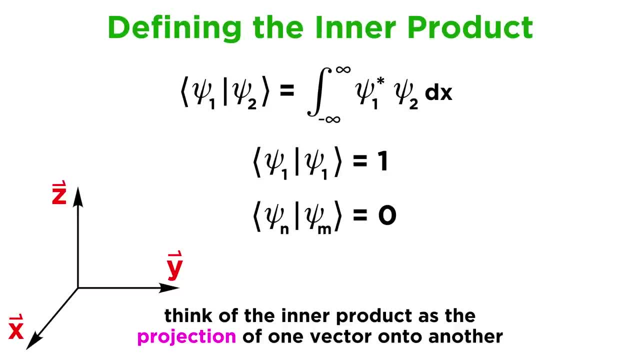 of the inner product as the projection of one vector onto another. Any orthogonal projection is zero, since we are dealing with linearly independent vectors, like how this unit vector in x does not contain any amount of the y or z vectors, But any projection of a vector 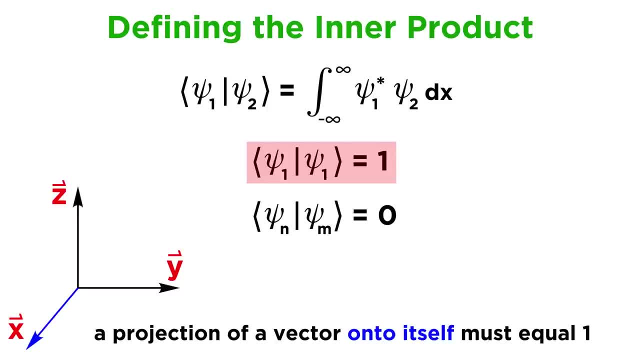 onto itself must be one, as a vector is equal to itself. The way to represent these relationships at the same time mathematically is to show the inner product of psi n and psi m as being equal to something called the Kronecker delta, which is presumed to be zero. 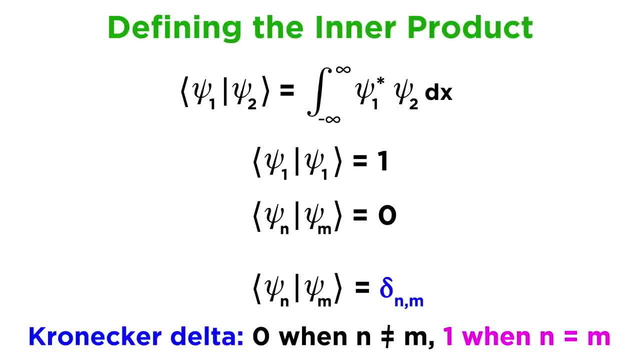 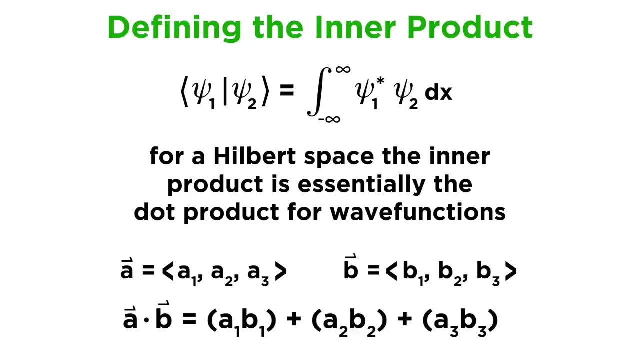 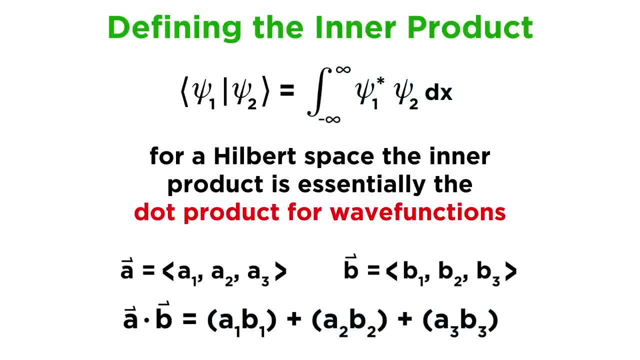 of two vectors from a vector space. So we can pretty much think of the inner product as the dot product for wave functions. The way we are using the dot product in this context is indeed the same as what we are familiar with, even though we are using integrals and functions rather than. 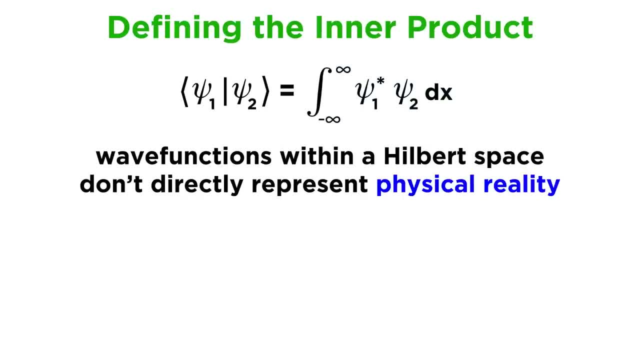 sums and vectors. It is simply that wave functions within a Hilbert space don't correlate with physical reality. Ket of psi is a vector in the Hilbert space, while psi of x is the projection of that vector onto the space we are familiar with such that we can describe observables. 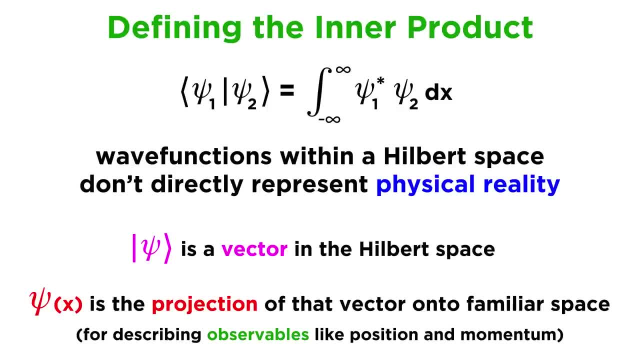 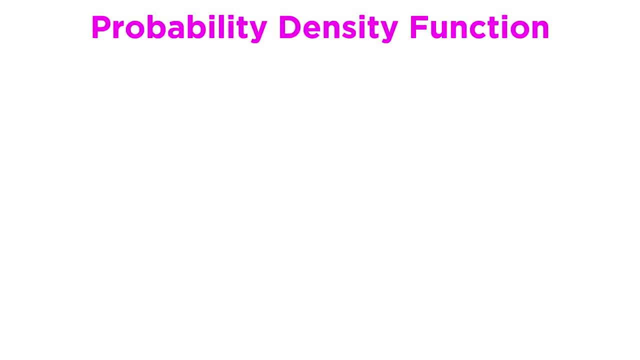 like position and momentum. With an enhanced view of the wave function, let's now return to the concept of the probability density function that we introduced in the previous tutorial. First, let's recall that the wave function is a vector of a vector space. 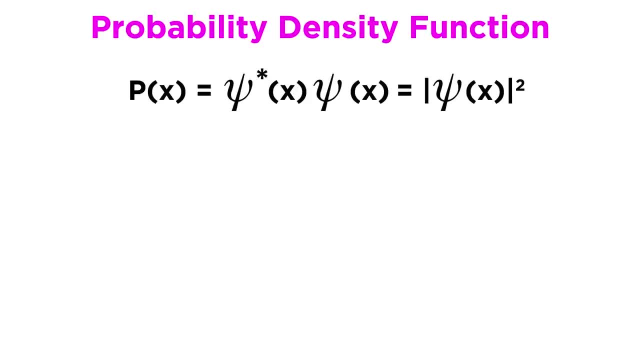 Let's recall the mathematical meaning of the probability density function with the following equation, involving the product of the wave function and its complex conjugate represented by psi star. So p of x equals psi, star times psi, which equals the absolute value of psi of x squared. Now let's expand a bit. The probability density function tells us that: 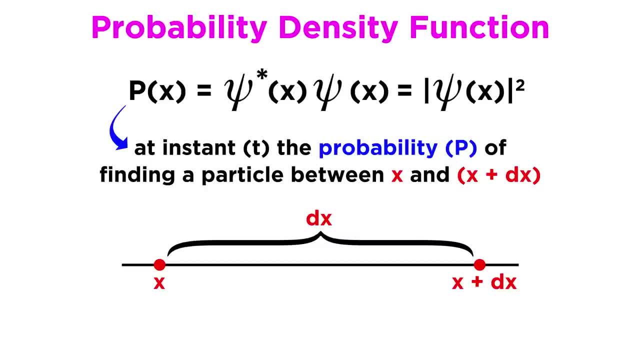 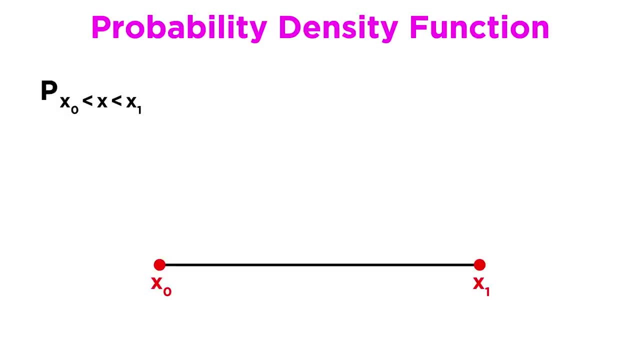 at some instant. t, the probability p of finding a particle between x and x, plus dx, is equal to psi, star times psi. We should note that the probability density is always a real number To find the probability that a particle will be found in some region. 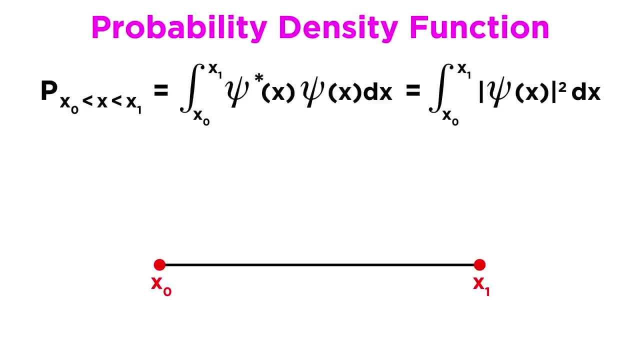 of space, we can calculate the following integral of the probability density function from x0 to x1.. Then let's understand that if we integrate the probability density function from negative infinity to positive infinity, then we can get the following integral. Let's: 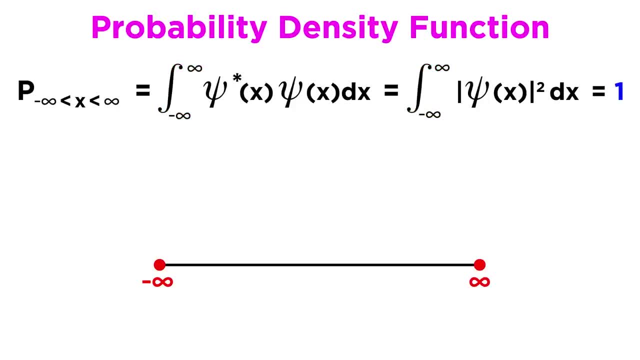 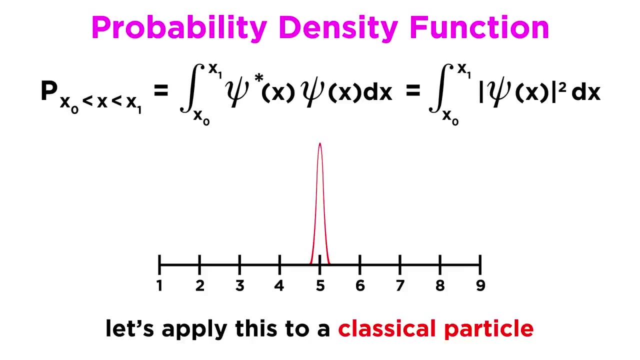 negative infinity to positive infinity, this will equal one, meaning that the probability of finding the particle somewhere in space is one hundred percent. If we were applying this to a classical particle, we would get a very narrow peak centered in a specific location. like x equals five, 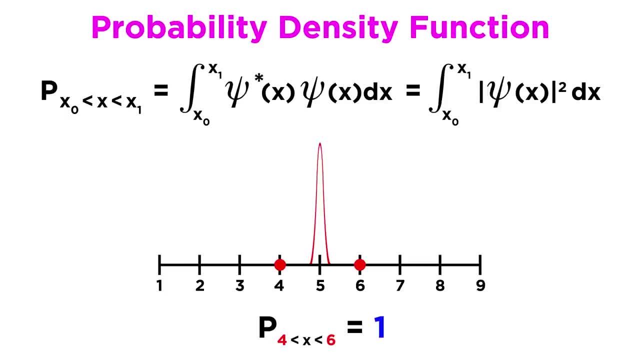 Integrating only from four to six, we would still get a result of one, since the particle is located within these boundaries. If we were to integrate over some other interval, we would get a result of zero, which makes sense, since the particle is not there but is somewhere else. 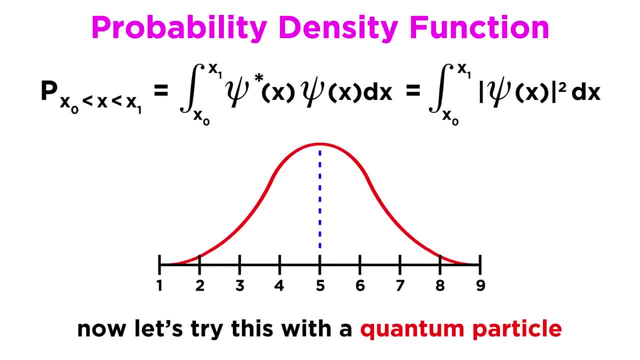 But with a quantum particle we get a different result. Perhaps it is still located at x equals five, but its presence is much more diffuse. In this example, the probability density function extends like a bell curve, let's say from one to nine. 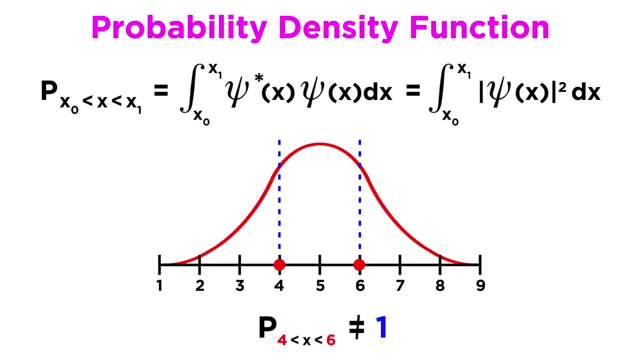 Integrating from four to six will no longer give us one. We will get some fraction of one, as will be the case with any other interval that contains some of the probability density function. Integrating over this interval will give us something close to one. let's say zero point. 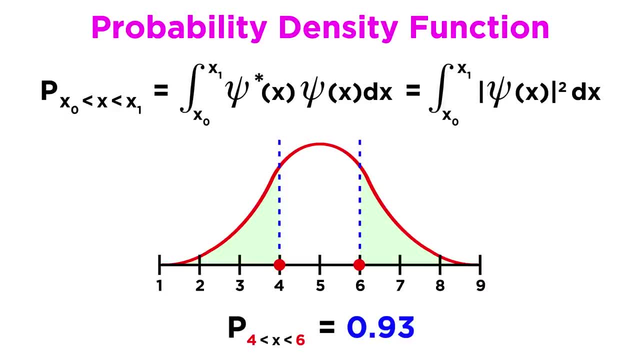 nine three, but there is still some probability, when performing a measurement, of finding the particle towards either edge of this bell curve. This is why normalization is so important. it ensures a result of one which is the equivalent of knowing with certainty that the particle is located within a particular boundary. 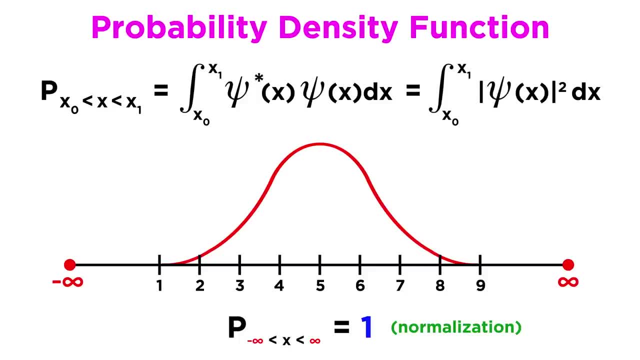 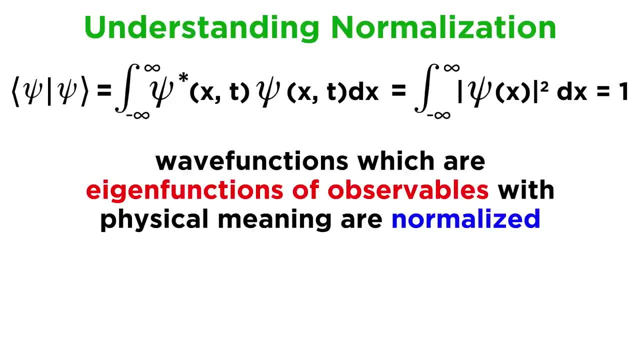 This means that the particle is located within a particular interval, because it's the largest possible interval: all space. It tells us that this particle exists, even though we don't know exactly where. Now we need to introduce some more terminology. We can say that wavefunctions, which are eigenfunctions of observables with physical meaning, are: 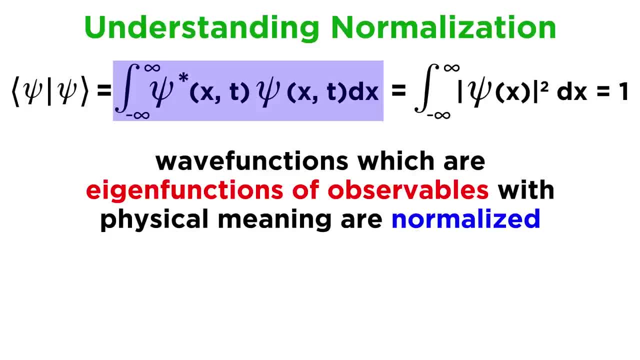 normalized Again. by normalized we mean that if we calculate the integral of the probability density function over all space, Which, as we know, is the integral over all space of the modulus squared of the wavefunction, it will always be precisely one. 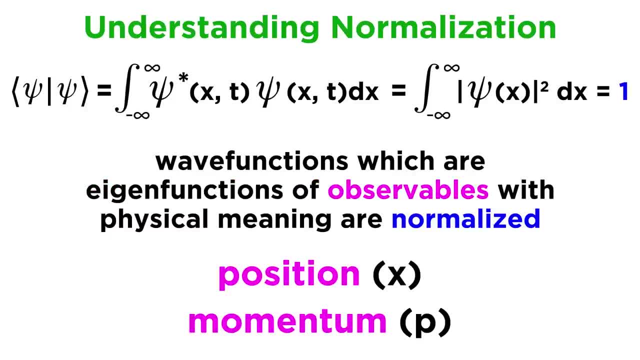 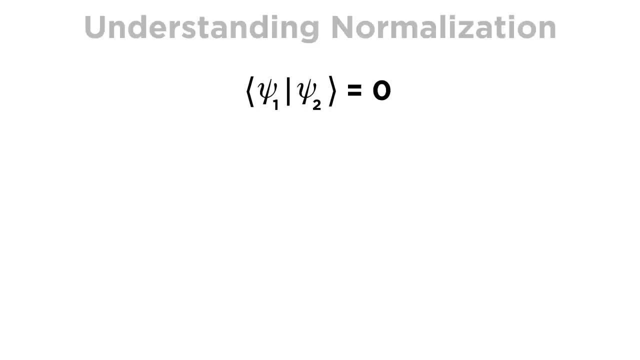 Rather predictably. two examples of observables with physical meaning that will have eigenfunctions in the form of normalized wavefunctions are position x and momentum p. In the next tutorial we will look at the inner product of psi and another wavefunction of the same vector, space. 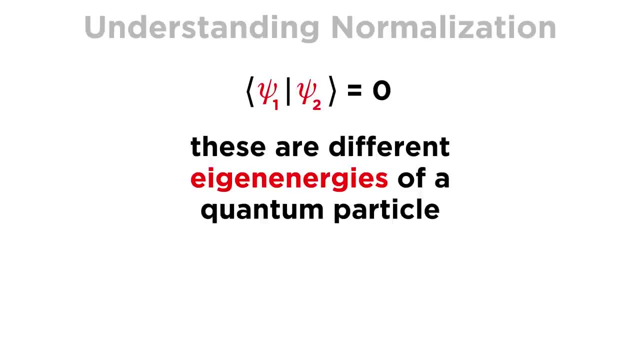 Like psi one, Psi two And so forth, which correspond to different eigenenergies of a quantum particle, And this will be equal to zero due to the linear independence of all wavefunctions forming such a vector space. But first let's continue to discuss normalization. 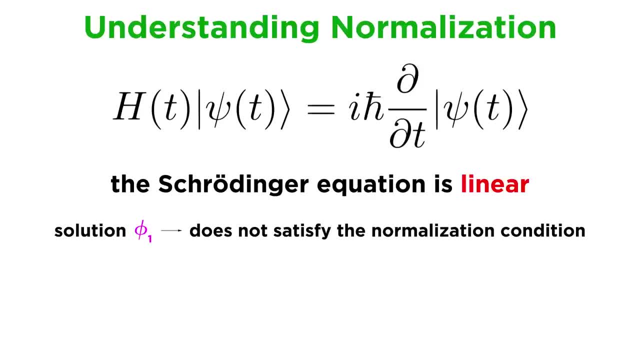 It is the case that the Schrodinger equation is linear, which means that, in finding a solution for this equation, if we arrive at a wavefunction, phi one- that doesn't satisfy the normalization condition, If of course the inner product of the wavefunction with itself does not equal one, but rather 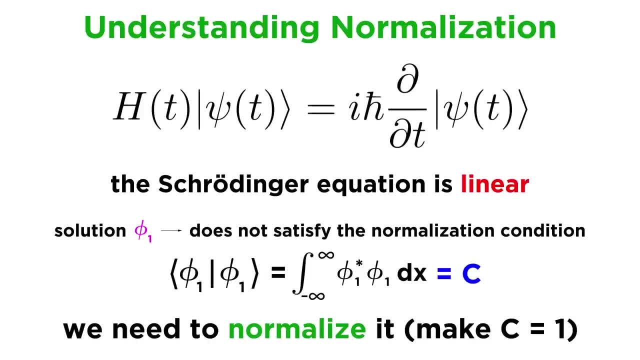 equals some constant c that is not equal to one, then we need to normalize it. We need to find a way to make c equal to one. Now it is the case that if a wavefunction is a solution to the Schrodinger equation, 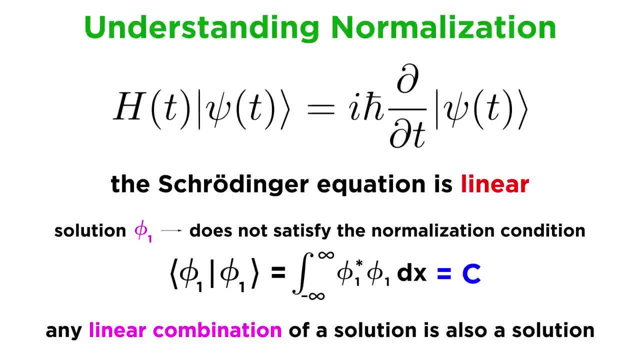 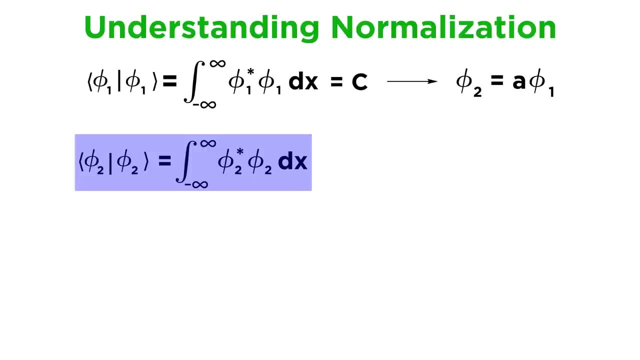 then any linear combination of this wavefunction will also be a solution. phi1 is a solution, then phi2, which is defined as equal to a phi1, must also be a solution. So since the inner product of phi2 with itself would look like this, we can also just replace: 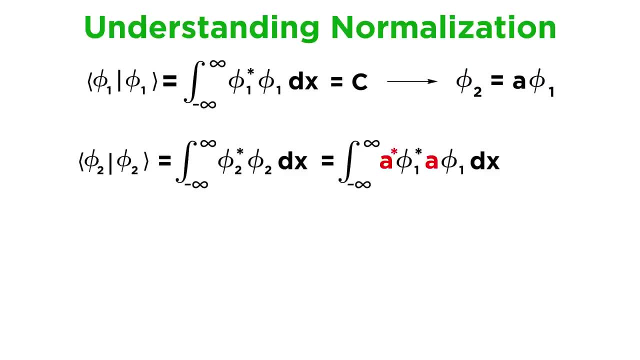 phi2 with a phi1, and we can then pull the constants a star times a out of the integral. This will equal 1. because we have decided that it should equal 1, because we need a normalized wavefunction and that is the condition of normalization. 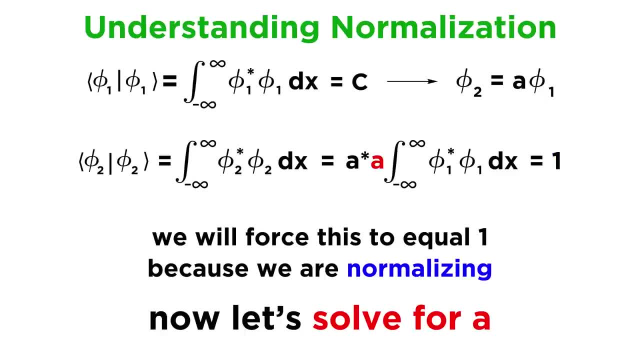 Now we can find what a must be for this to be true. So recall that the expression for phi1 gave us a value of c. Let's therefore replace this entire integral in the previous expression with c, since they are equivalent. That gives us a star times a times c equals 1.. Recalling that a star times a equals the absolute value of phi1,, we can then replace phi1 with a star times a times c equals 1.. Recalling that a star times a equals the absolute value of phi1,, we can then replace phi1 with: 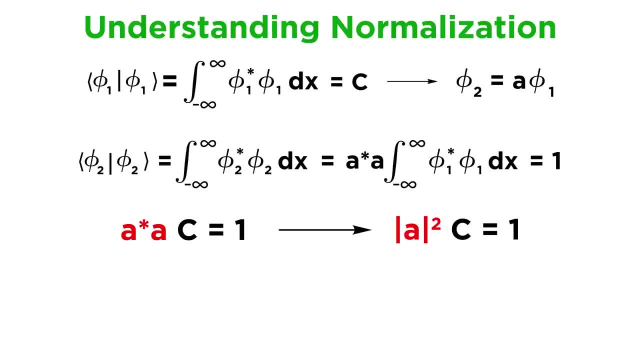 a star times a times c equals 1.. Recalling that a star times a equals the absolute value of a quantity squared. since these terms differ only in the sign of their imaginary terms, we can then divide both sides by c. take the square root, and a will be equal to 1 over root c, where c represents the inner. 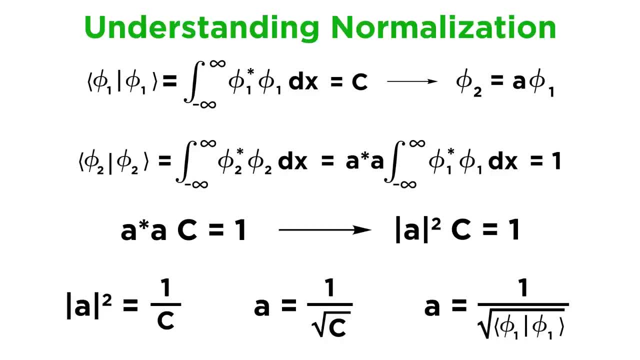 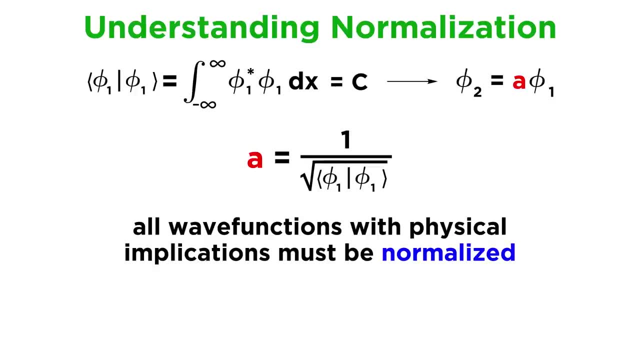 product of phi1 with itself. The main thing we should take from all this is that all wavefunctions with physical implications must be normalized. In other words, the definition of the probability density must be normalized. The definition of the probability density function implies that wavefunctions which 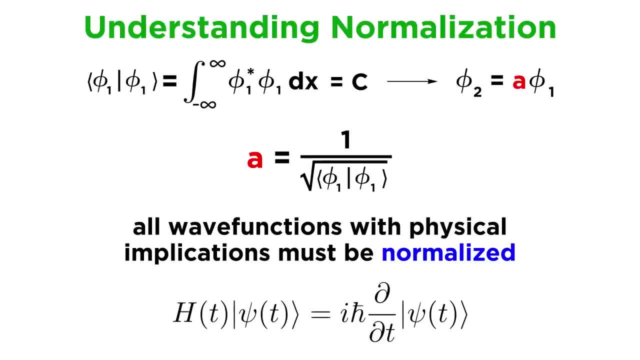 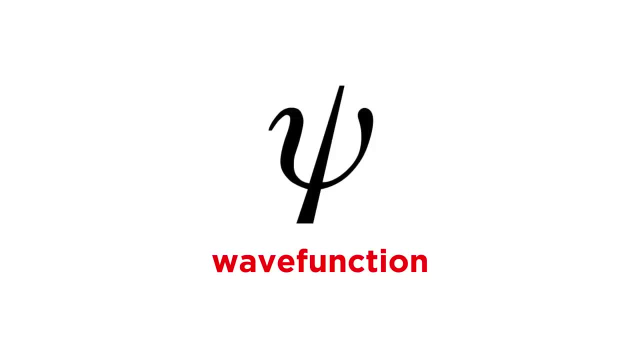 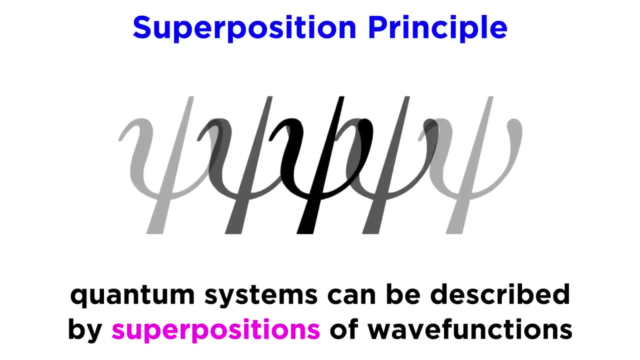 are solutions of the Schrodinger equation must be normalized, and we will talk more about the Schrodinger equation in the next tutorial. Now that we have a better understanding of wavefunctions, let's see what we can do with them. First, let's talk about the superposition principle. 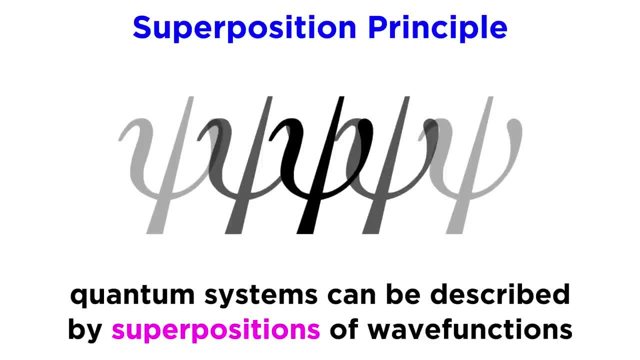 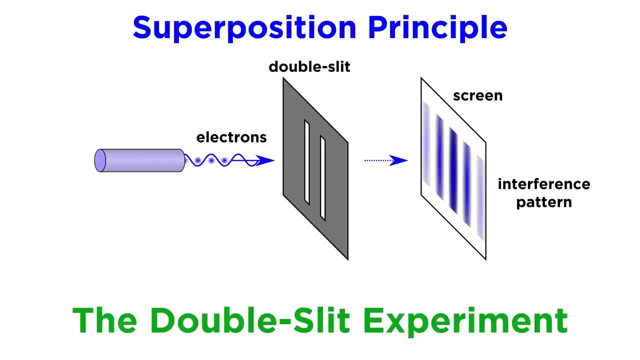 This states that quantum systems can be described by combinations or superpositions of wavefunctions which still must satisfy the norm. One example of this is the famous double-slit experiment, which we introduced on a conceptual level in a previous tutorial. Now let's add some math. 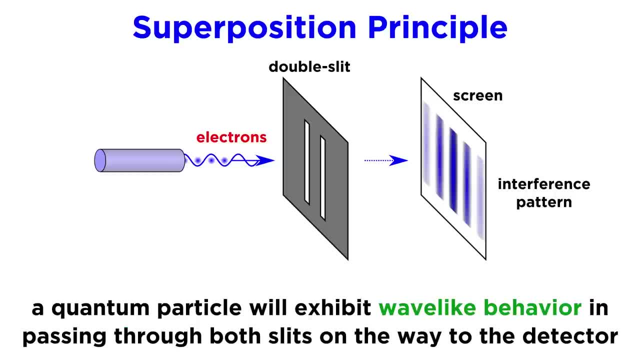 As we recall, given this, grating with two slits, a quantum particle will exhibit wave-like behavior, passing through both slits and generating an interference pattern at the detector. beyond, The interesting feature of this experiment is the act of the particle passing through: 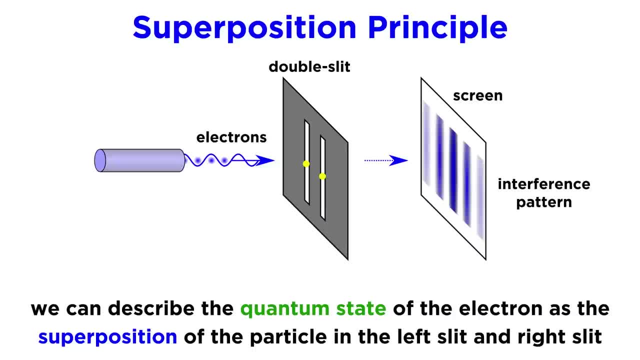 both slits simultaneously. At this moment, we can describe the quantum state of the particle as the superposition of the particle being in the left slit and the particle being in the right slit. Mathematically, we would represent this as psi equals phi L plus phi R, essentially representing 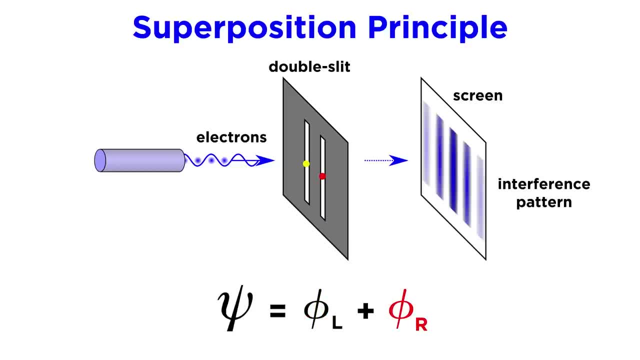 the sum of a wavefunction localized at one slit and a wavefunction localized at the other. Now let's introduce two constants, aL and aR, which represent the probabilities of the particle being at either slit. If we desired, we could make this more complicated by adding more slits, and in turn we would. 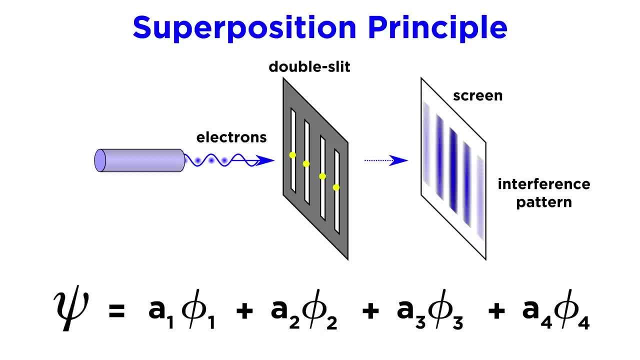 simply add more wavefunctions to this equation, each with their own respective constant. If there were four slits, we would describe the superposition this way: with four wavefunctions and four constants, where phi one represents the wavefunction of a particle at slit one. 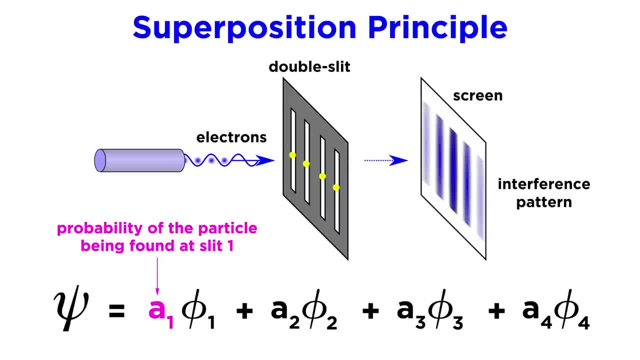 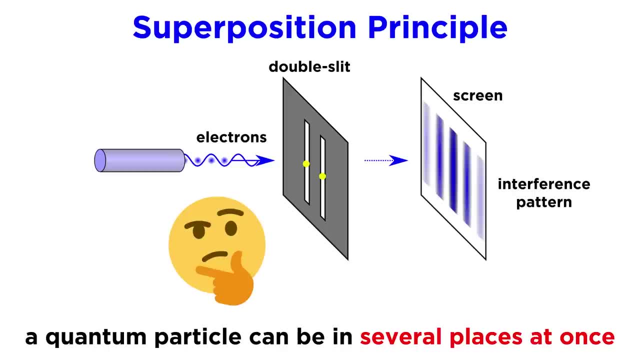 and a one represents the probability of the particle being found at slit two. Now let's look at this again At slit one And the same for the other three. What we must wrap our heads around as best we can is that the superposition tells us. 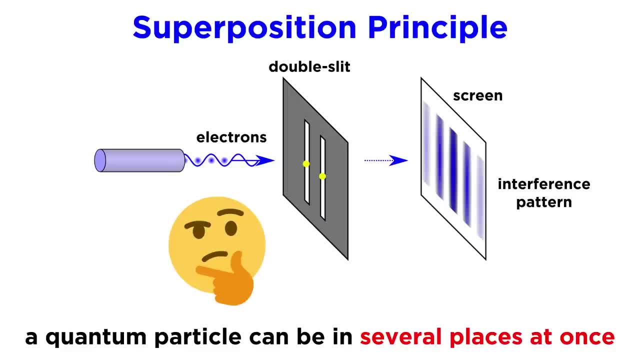 that a particle can be at several points at the same time, and this is precisely what the double-slit experiment demonstrates, as the particles do physically pass through both slits. It is a probabilistic way of viewing reality that is difficult for our classically trained. 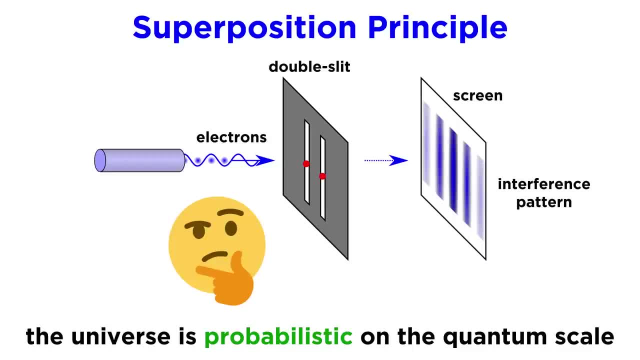 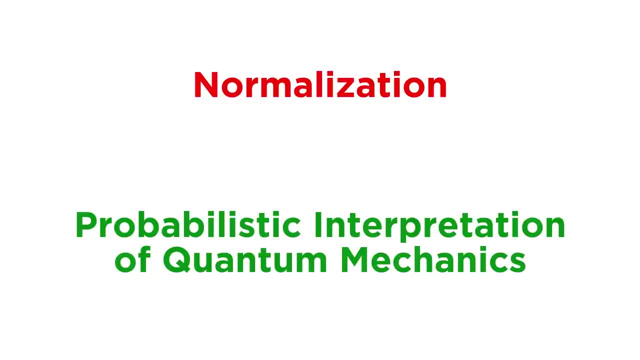 brains to comprehend, but nevertheless, this is how the universe operates automatically. But nevertheless, this is how the universe operates automatically, And this is precisely what the double-slit experiment demonstrates as the particles operate on this scale. Now that we understand normalization and the probabilistic interpretation of quantum mechanics, 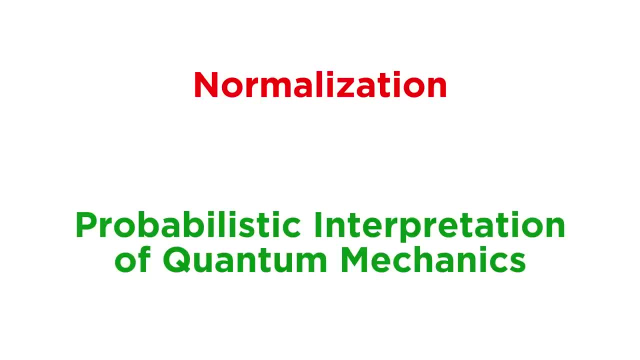 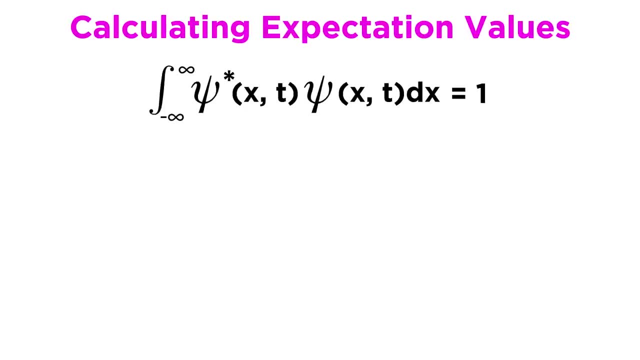 we are ready to develop one of the most important topics in quantum mechanics, and that is the calculation of expectation values. Earlier we saw that the integral over all space of the probability density function gives us a value of one for a normalized wavefunction. This one, which is the maximum value possible, tells us that the probability density function 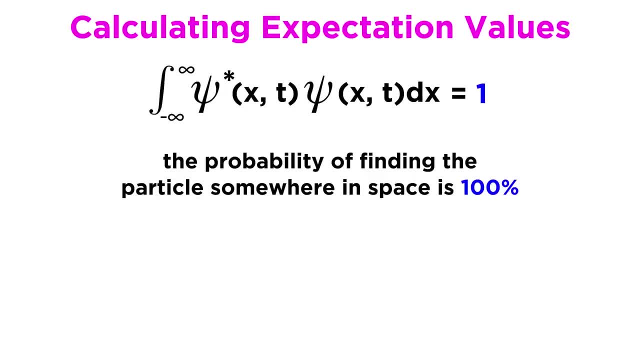 is one. This tells us that the probability of finding the particle somewhere in space is 100%, which makes sense, since the particle has to exist somewhere. Now, if we want to determine where it is most likely to find the particle, we have to perform. 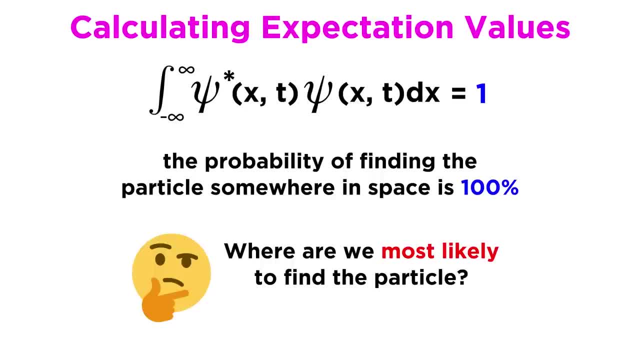 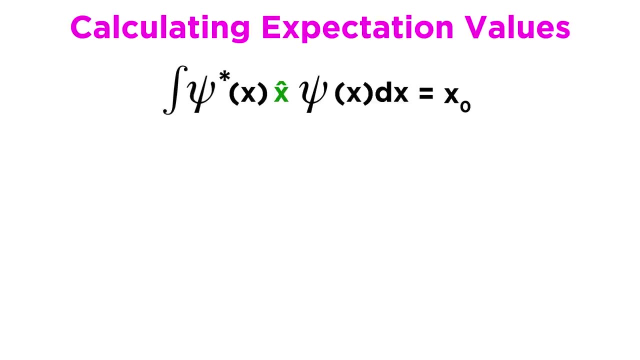 a similar calculation. Given that we are talking about the location of the particle, we are describing its position, so we will need to use the position operator in conjunction with the probability density function. The operator will be placed like so: in between psi star and psi, such that it acts on psi and this expression will. 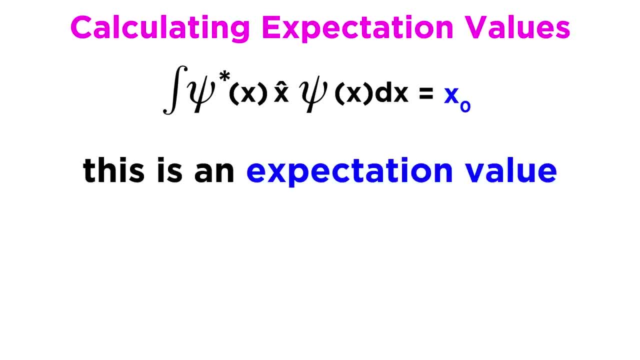 be equal to x zero. X zero is an expectation value. It is a number which, in this case, tells us the most probable location of the particle. Now let's try to understand this in greater detail. In statistics, an expectation value is a weighted average of a variable. 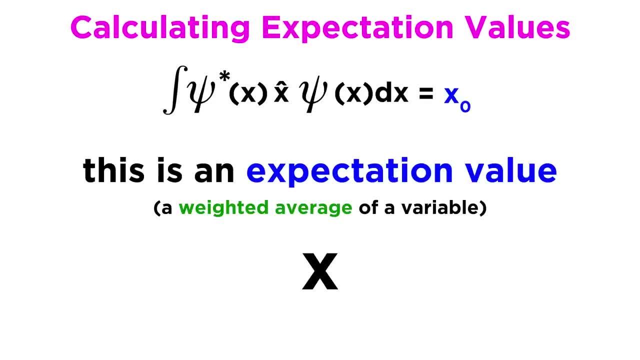 Think of it this way. Consider the variable x, but it does not have a definite value. It exists as a distribution of values, something which will be true all the time. in quantum mechanics, as we are beginning to understand, The expectation value is the weighted sum of all possible values. that x can take times. 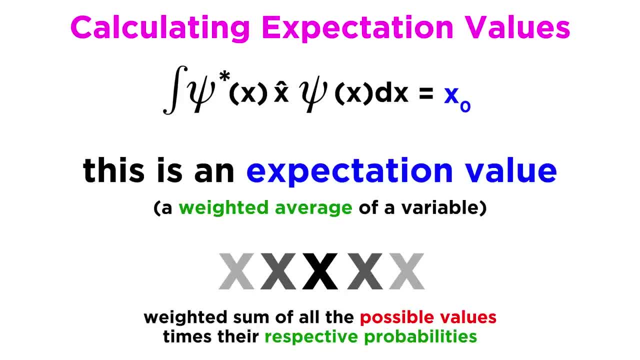 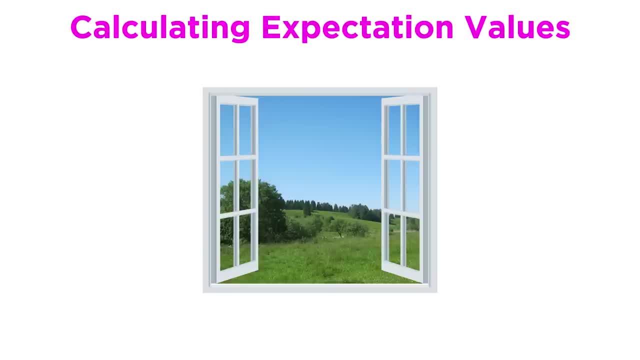 their respective probabilities. so each value contributes to the sum in a way that is proportional to its respective probability. Now let's apply this to quantum mechanics, Say. we are performing an experiment. many, many times Perhaps we are throwing a quantum particle out the window such that it lands on the 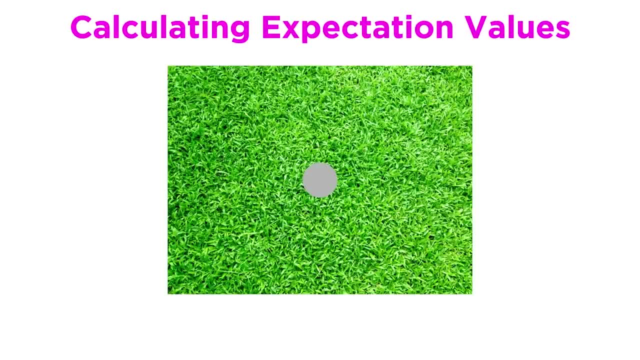 ground below and we take a picture of where it lands each time, Then say we superimpose all of the pictures for all the trials so that we can see all of the final positions at once and whenever it lands in the same spot again that spot. 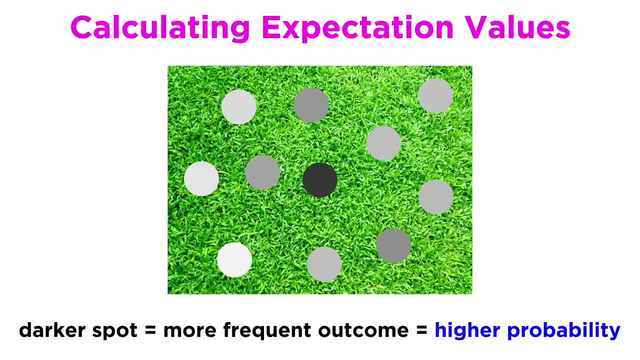 becomes darker. This singular image tells us the most probable position for the particle, with the darkness of each spot relating to x, And we can consider the darkest spot to be representative of the expectation value for position at the measuring device which, in this case, we are analogizing to be the ground. 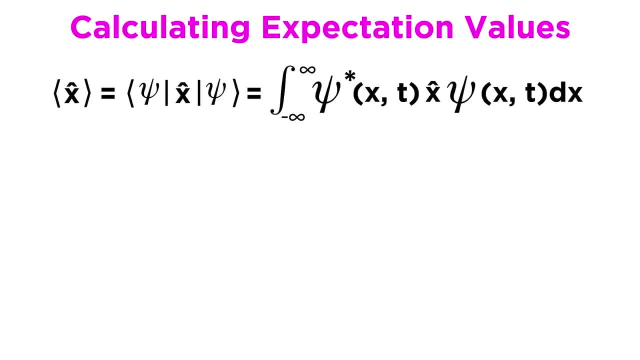 itself. Once again, mathematically, we will write this as the integral over all space of psi star times, the position operator acting on psi. This is how we define the expectation value of the x-coordinate at a given point in time. We can also write this as the integral over all space of psi star times, the position operator. 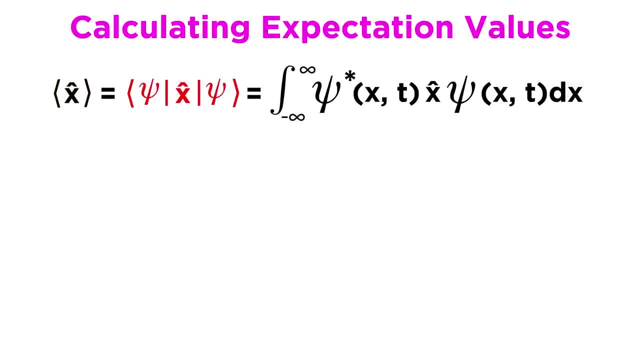 acting on psi. This is how we define the expectation value of the x-coordinate at a given time, t, which is written this way and read as the expectation value of x with wavefunction psi. Notice how we use both left and right brackets, with the variable in the middle. 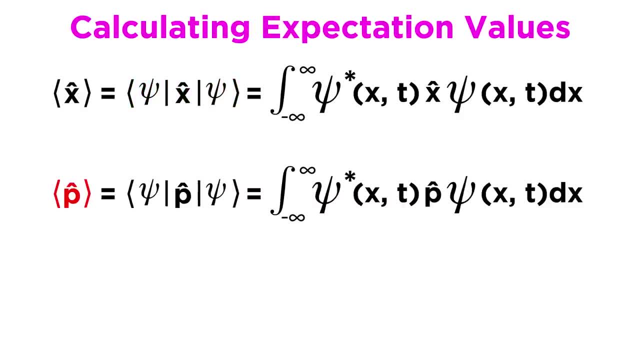 We can write an equivalent equation for the momentum operator, whereby the expectation value of p equals the integral over all space of psi conjugate times the operator p acting on psi. We can then rewrite this. This is all determined using the definition of the momentum operator which, as we recall, 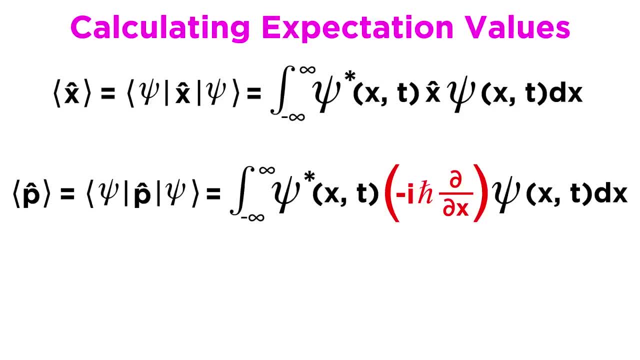 from the previous tutorial is negative. I times H-bar, times the partial derivative with respect to X. This applies in a broader context as well. We can write all dynamical variables as functions of position and momentum. This means that it is possible to find the expectation value of any dynamical variable. 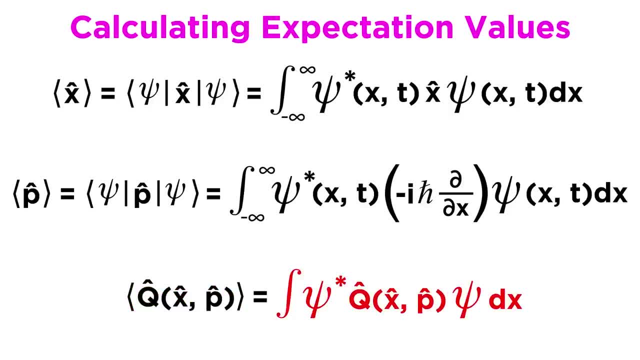 q by calculating it this way, with the expectation value of q of xnp being a negative number point of the x-coordinate p, where a simple f ان xnp is equal to a integral over all space of, seems to be right. So this is great. It is still a tip, but we can still do some tomorrow. Thank you so much for joining us. I am Dan Stinfield, for paused каж singlené thinné szeno. I am essentially Dan St functioning here. 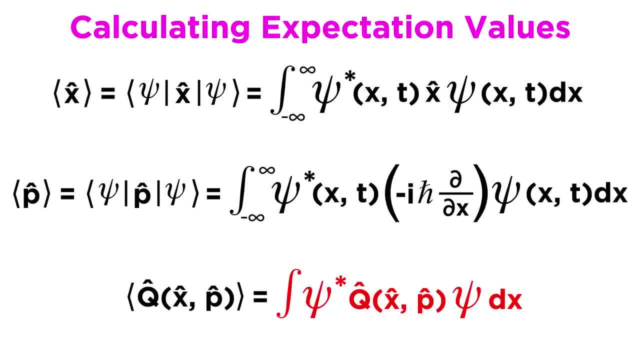 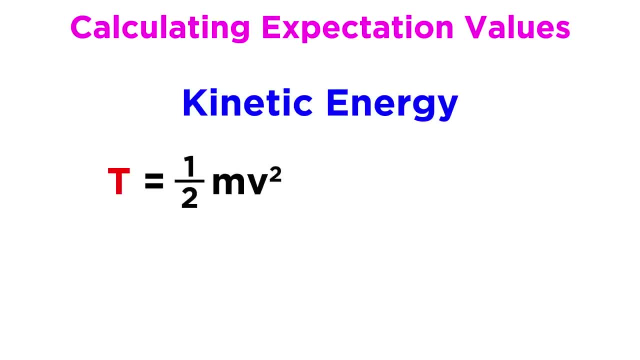 I am Dan Stinfield Bye being equal to this expression. Let's apply this to one specific example: kinetic energy. In the classical physics series, we learned that the kinetic energy of an object, which from now on we will represent as t, is equal to one half mv squared. 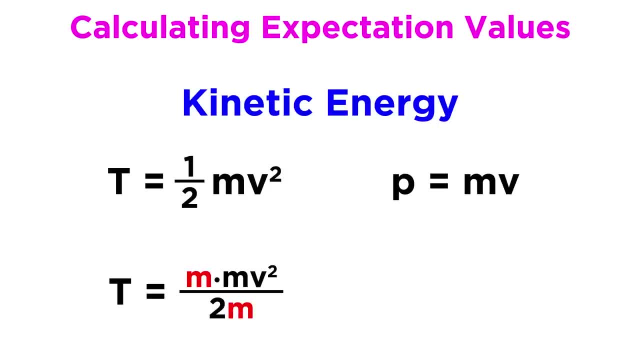 And since momentum equals mass times velocity, if we just put an additional mass term in both the numerator and denominator to keep the expression equivalent, we can change m squared, v squared into mv, quantity squared or p squared, leaving us with p squared over 2m. 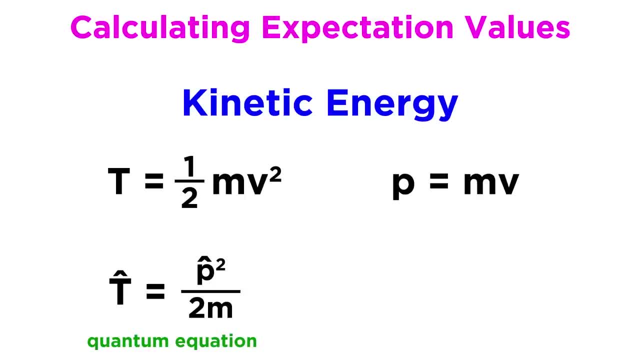 Now we can take this classical equation and translate it into a quantum equation by replacing momentum with the momentum operator. Let's then plug in our expression for the momentum operator, putting it out front, but twice, Since the operator is squared. Now, to simplify: negative i times, negative i gives i squared, or negative one. so let's 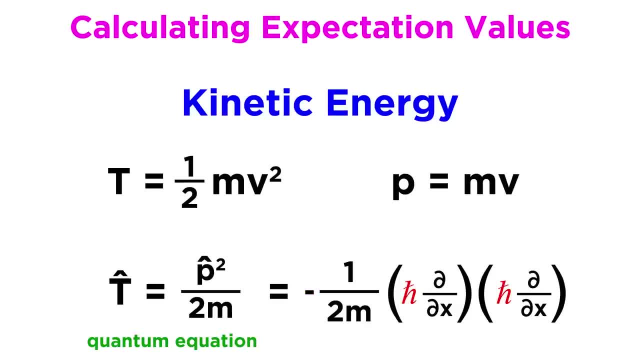 just get rid of those and make the whole expression negative. Then we can pull h bar squared up here and the partial derivatives multiply to give the second derivative with respect to x. This is the quantum operator for kinetic energy which we will be using frequently. 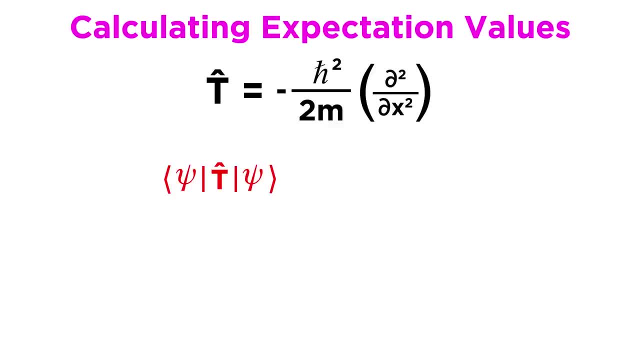 Now let's find the expectation value for the momentum operator. This is the equation value for kinetic energy for a given wavefunction, psi. As we learned to do this, we place the operator T in between the bra of psi and ket of psi. 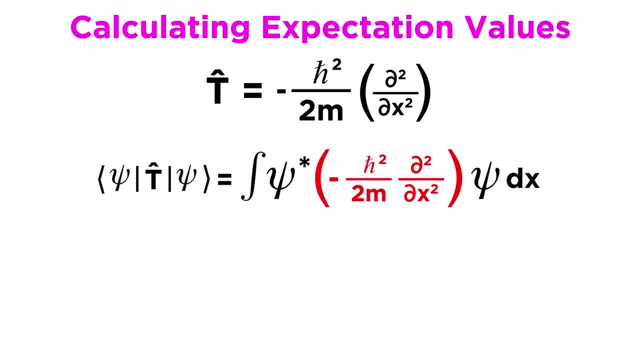 We can then replace the operator with the expression it represents. We get the integral of psi star times, the kinetic energy operator, acting on psi dx. Recall that, even though we are not writing it explicitly. psi depends on x, which is why we are able to differentiate it with respect to x. 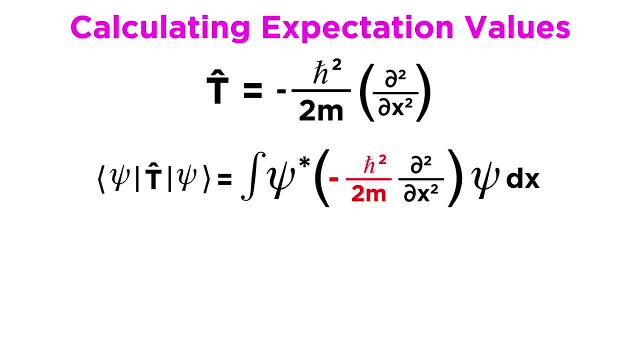 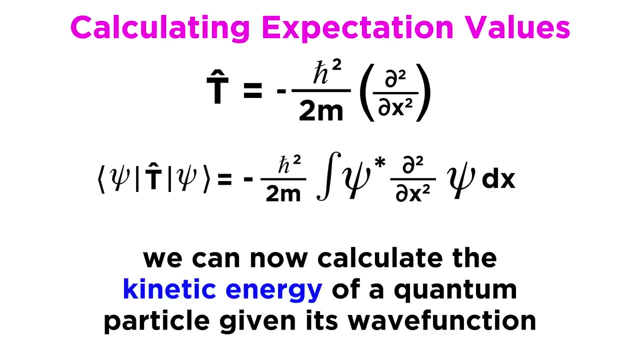 Now recognize that we have some constants with h, bar and mass. so let's pull all of this out of the integral. That leaves psi, star times, the second derivative of psi, with respect to x, dx. So we can now calculate the kinetic energy of a quantum particle given its wavefunction. 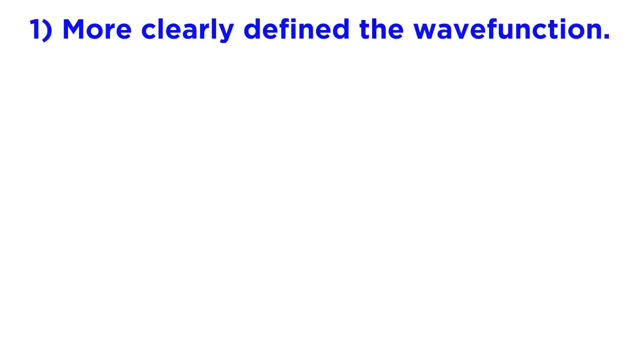 In this tutorial, we did several things. First, We more clearly defined what a wavefunction is, from both a conceptual and mathematical standpoint. We learned that wavefunctions are a special type of vector living in something called a Hilbert space. Next, we outlined the most important properties of wavefunctions, namely that a quantum system,